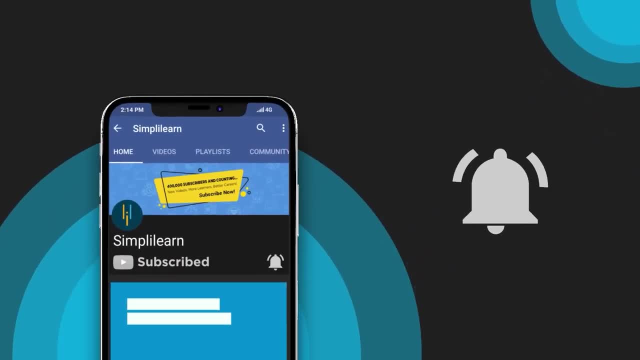 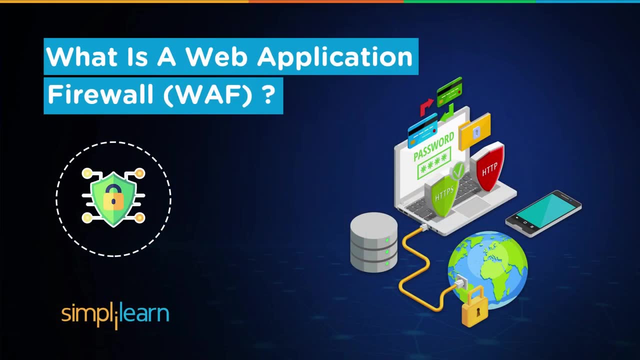 Welcome back to our channel. I am Abhisar, and today we are delving into a crucial aspect of web security that safeguards our online experiences: the web application firewall. In this video, we will unravel the mysteries of what a web application firewall is, how it works and why it's a vital defender against cyber threats. 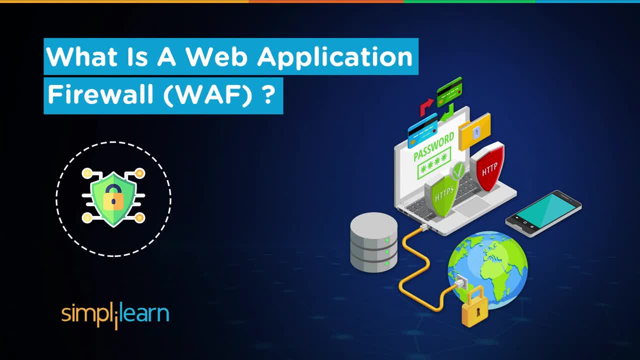 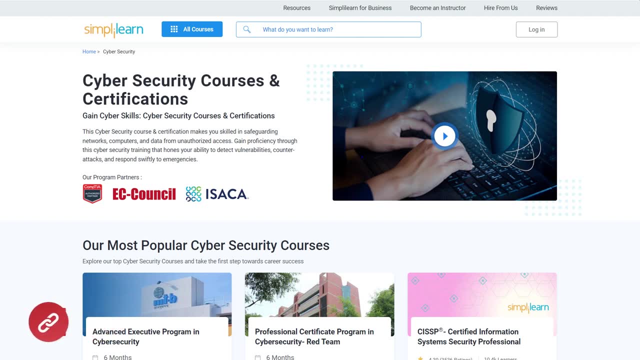 Whether you are a tech enthusiast or just curious about online security, you are in the right place. So let's dive in. And just a quick info for you: if you want to upskill yourself, master cybersecurity skills and land your dream job, 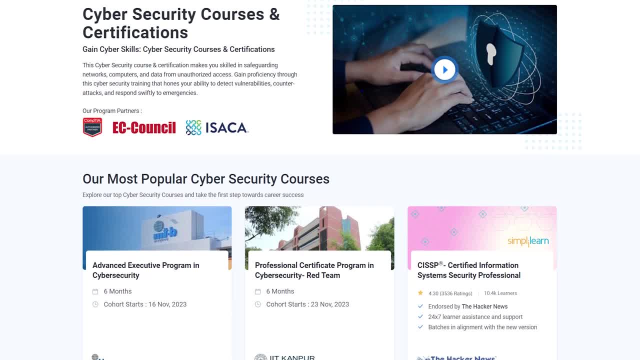 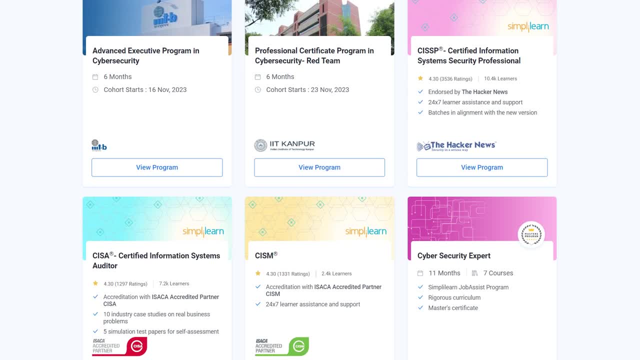 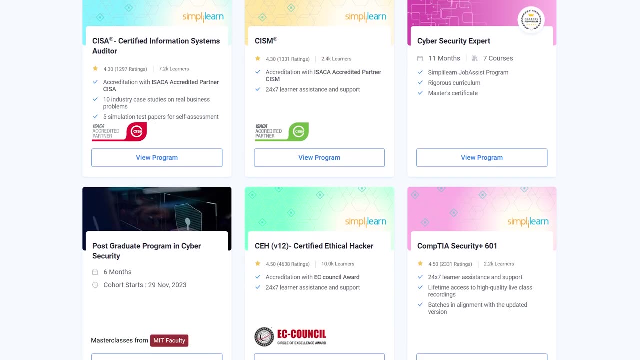 or grow in your career, then you must explore Simply Learn's cohort of various cybersecurity programs. Simply Learn offers various certification and postgraduate programs in collaboration with some of the world's leading universities like MIT, IIT, Kanpur, EC, Council and many more. Through our courses, you will gain knowledge and work-ready expertise. 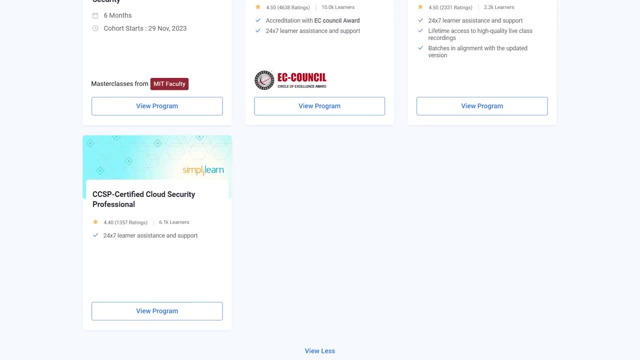 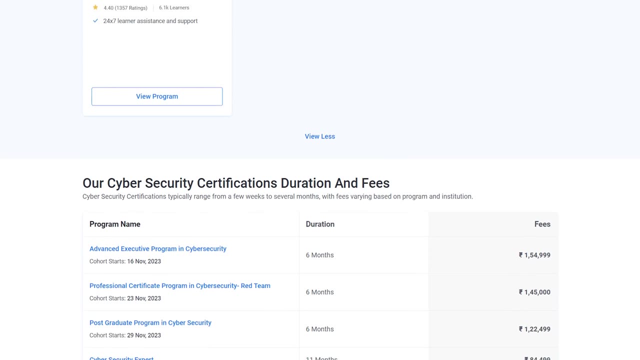 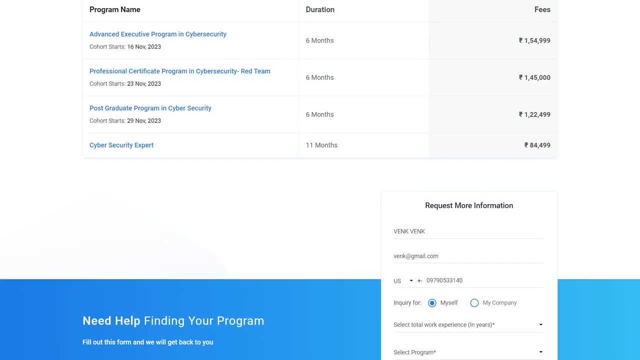 in skills like advanced hacking concepts, network packet analysis, ethical hacking, network security and over a dozen others. That's not all. you also get the opportunity to work on multiple projects and learn from industry experts working in top-tier products and security companies and academicians from top universities. After completing these courses, 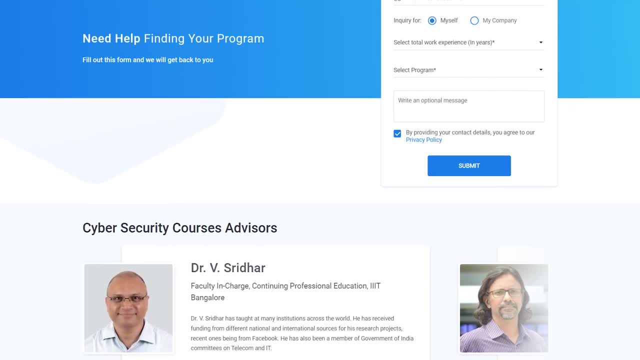 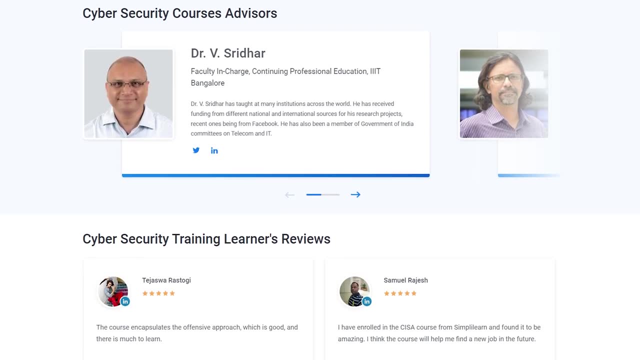 thousands of learners have transitioned into a cybersecurity role as a pressure or move on to a higher paying job or profile. If you are passionate about making your career in this field, then make sure to check out the link in the pinned comment and description box. 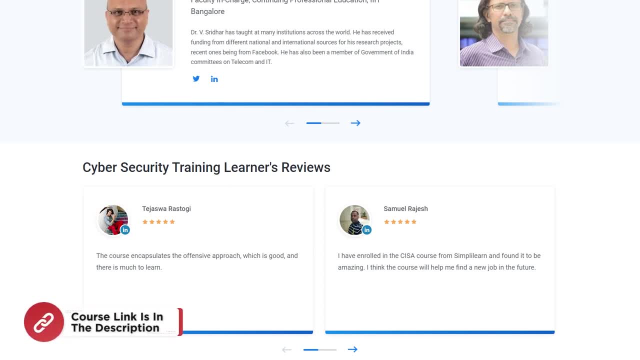 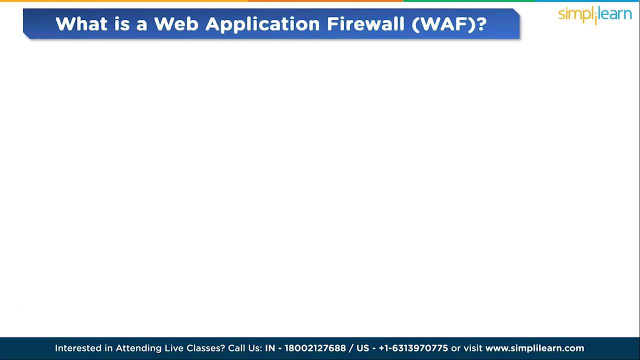 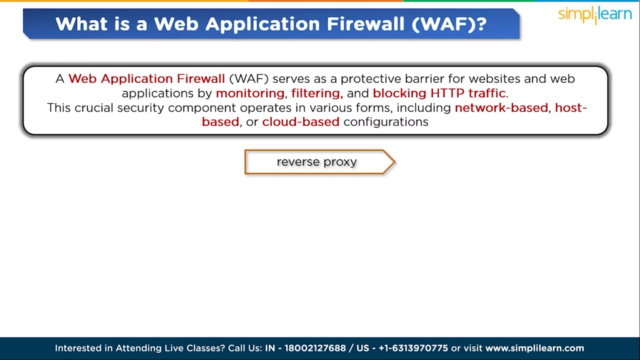 to find a cybersecurity program that fits your experience and areas of interest. So let's get started, And here we'll start with what is a web application firewall? So a web application firewall serves as a protective barrier for websites and web applications by monitoring, filtering and blocking HTTP traffic. 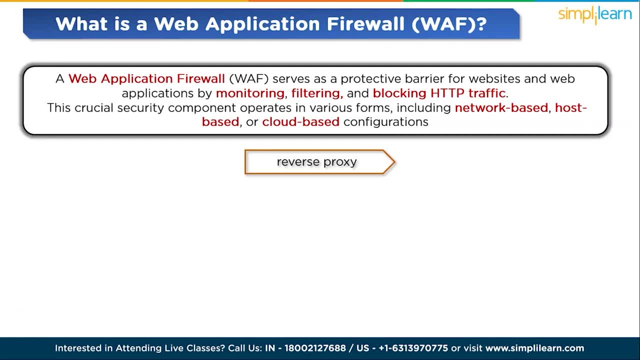 This crucial security component operates in various forms, including network-based, host-based or cloud-based configurations, Typically deployed via a reverse proxy. the WAF is strategically positioned in front of one or more websites or applications, Whether functioning as a network appliance, server plugin or cloud service. the WAF meticulously examines. 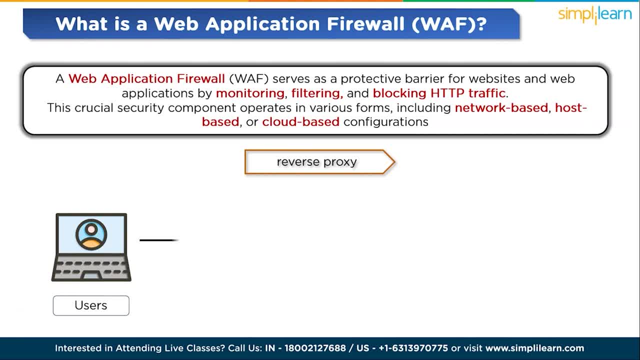 each packet. It employs a rule-based approach to scrutinize layer 7 web application logic, identifying and filtering out potentially harmful traffic that could exploit vulnerabilities. Enterprises commonly leverage web application firewalls as a fundamental security measure. Their role is vital in safeguarding web systems against a spectrum of threats. 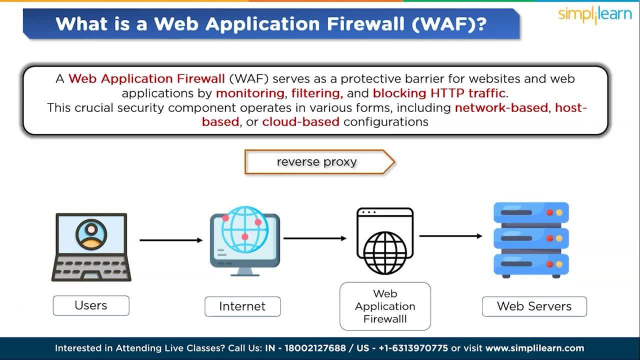 including zero-day exploits, malware infections, infestation and both known and unknown vulnerabilities. And one notable strength of WAFs lies in their ability to conduct customized inspections, swiftly detecting and preventing critical web application security flaws. And businesses offering products or services online, such as e-commerce platforms or online. 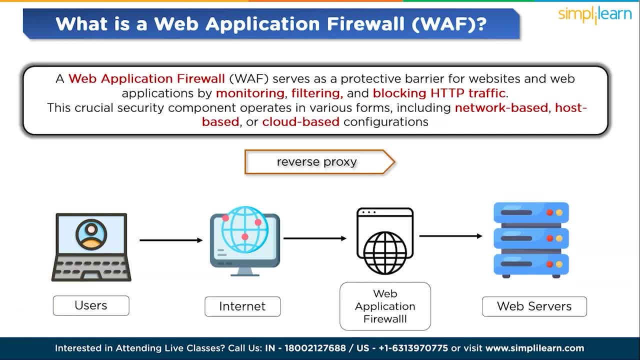 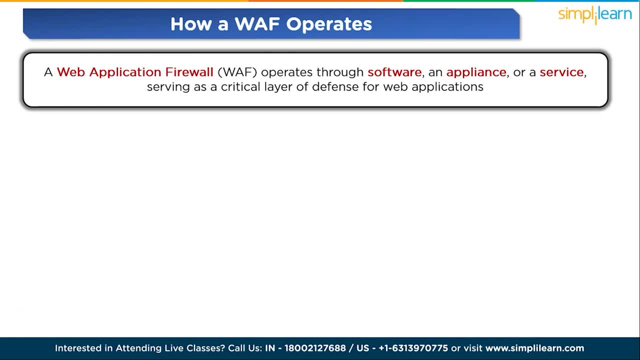 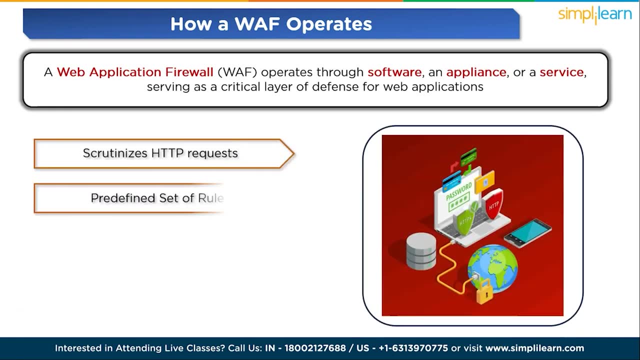 banking services find WAFs particularly advantageous. Now we'll see how a WAF operates. A web application firewall operates through software, an appliance or a service serving as a critical layer of defense for web applications. It meticulously scrutinizes HTTP requests, employing a predefined set of rules to distinguish between harmless 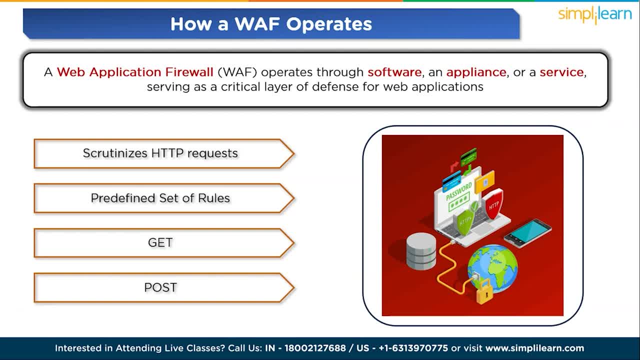 and malicious elements within the communication. The core elements of HTTP conversations subjected to WAF analysis predominantly include GET and POST requests. GET requests are employed for data retrieval from the server, while POST requests facilitate the submission of data to a server for altering its state. The WAF, in essence acts as a gatekeeper. 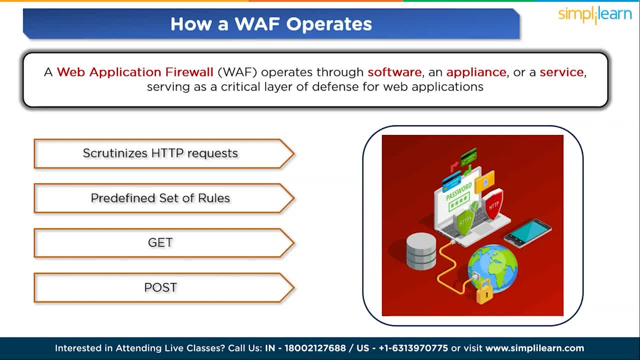 intelligently discerning and filtering the content of these requests, based on its toolset to ensure the security and integrity of web applications. This dynamic process allows the WAF to proactively identify and mitigate potential threats, such as SQL injections and cross-site scripting attacks, contributing to a robust defense against a myriad of. 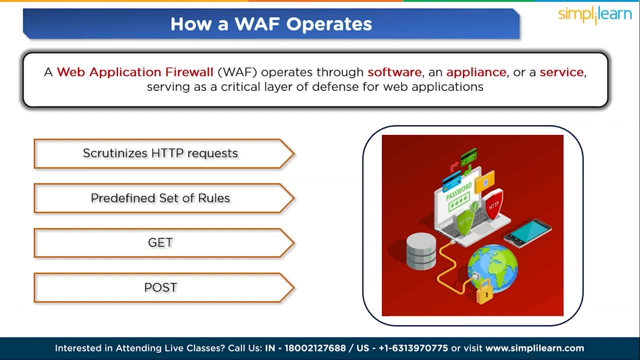 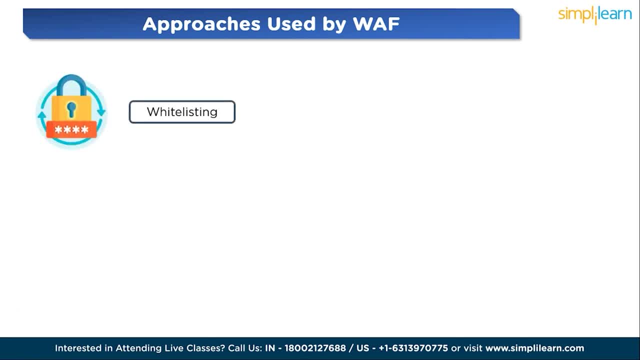 web application vulnerabilities. And now we'll move to approaches used by WAFs. So WAF employs various approaches to analyze and filter content within HTTP requests, and these methodologies include white listing. that is number one, and here WAF adopts a default. 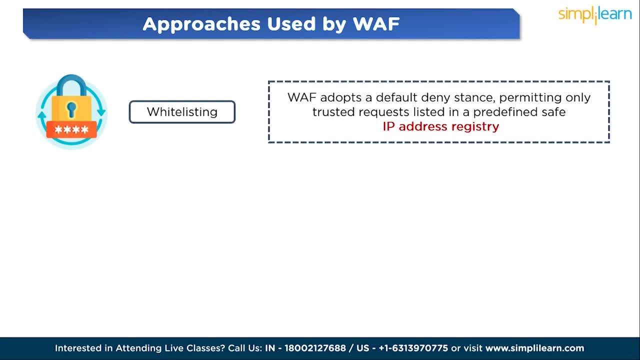 deny stance, formatting only trusted requests listed in a predefined safe IP address registry. White listing is a resource efficient compared to black listing, but may inevitably block legitimate traffic due to its broad filtering approach. While it offers efficiency, precision may be compromised. And then comes black listing Utilizing preset signatures. 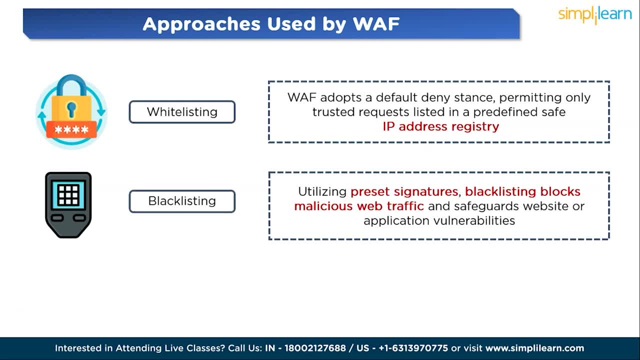 black listing blocks malicious web traffic and safeguards website or application vulnerabilities. It employs a set of rules to identify malicious packets, making it suitable for public websites handling traffic from unfamiliar IP addresses. White listing is resource intensive and requires detailed information to filter packets based on specific characteristics rather than relying on trusted IP addresses. 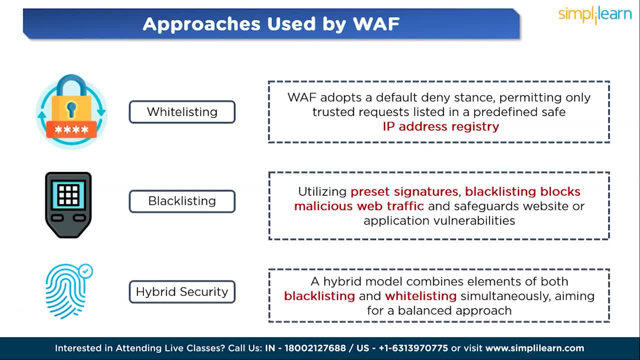 And then comes hybrid security. A hybrid model combines elements of both blacklisting and whitelisting, simultaneously aiming for a balanced approach. This model seeks to leverage the strength of both methods, providing a more nuanced and adaptive security strategy, Regardless of the chosen security model. WAF's scrutiny of the security model is very important, as it is the only security model in the world. WAF's scrutiny is very important as it is the only security model in the world. Regardless of the chosen security model, WAF's scrutiny of the model is very important, as it is the only security model in the world. It is also important to minimize HTTP interactions. 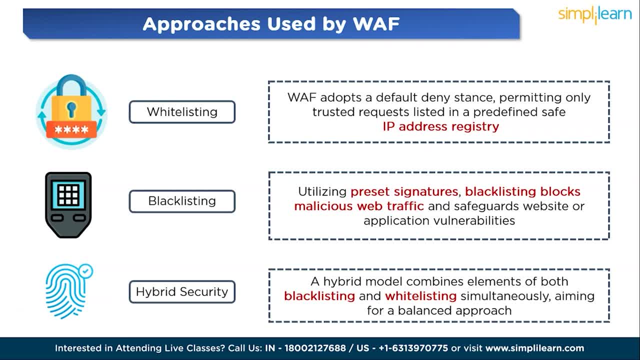 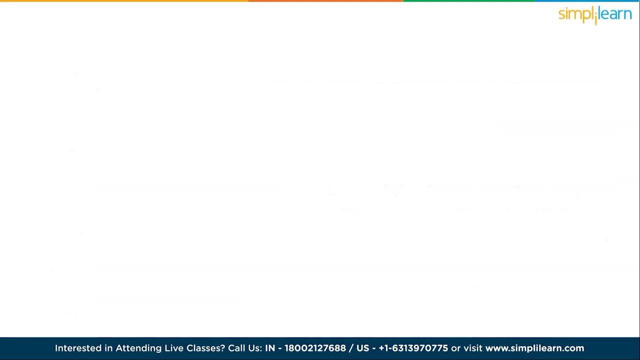 preemptively, mitigating malicious activity before reaching the server for processing. Regular policy updates are crucial for addressing emerging vulnerabilities, although some WAFs now incorporate machine learning for automatic updates. And then comes the importance of web application firewalls in modern expertise. In the ever-expanding digital landscape, web application firewalls play a crucial role in 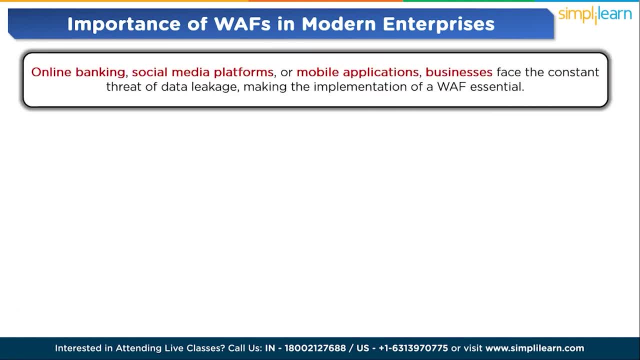 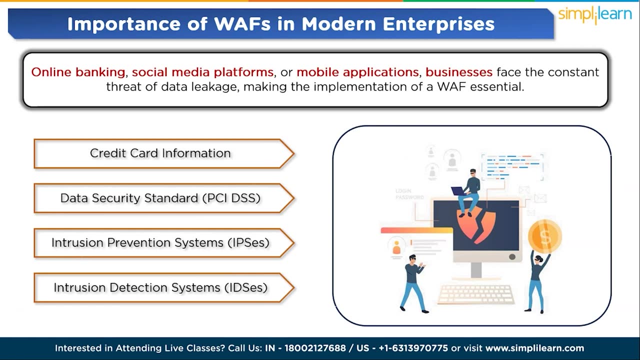 empowering many open artificial intelligence enterprises offering online products and services, Whether it's online banking, social media platforms or mobile applications. businesses face the constant threat of data leakage, making the implementation of a WF essential. One primary concern is the protection of sensitive data like credit card information and customer records. 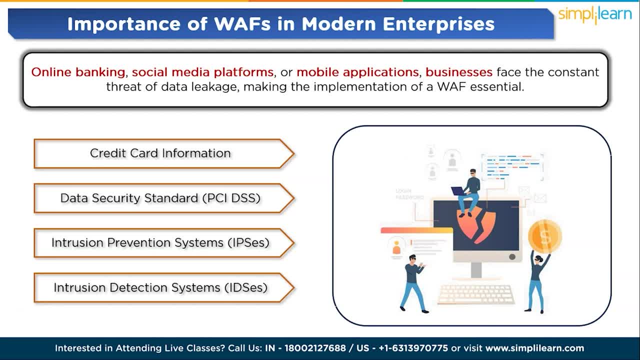 Often stored in backend databases accessible through web applications, And cyber attackers frequently target these applications to exploit vulnerabilities and gain unauthorized coverage. unauthorized access to valuable data and for industries like banking and compliance with standards such as the payment card industry data security standard PCI DSS is paramount. a WAF becomes a valuable asset in meeting PCI. 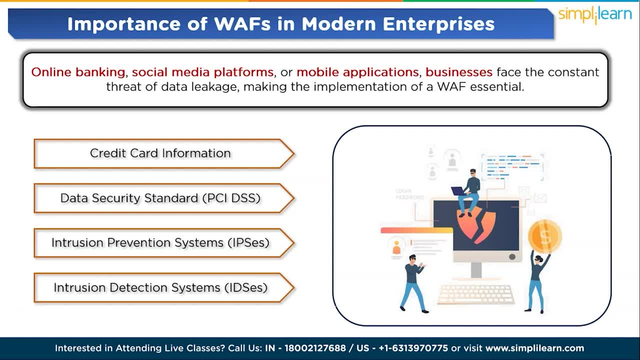 DSS requirements, specifically the mandate for a robust firewall system. as enterprises increasingly adopt mobile applications and engage in transactions by the Internet of Things, the application layer becomes a prominent arena for potential security breaches. if the WF emerges as a cornerstone in the modern business security model, however, it's crucial to recognize that the 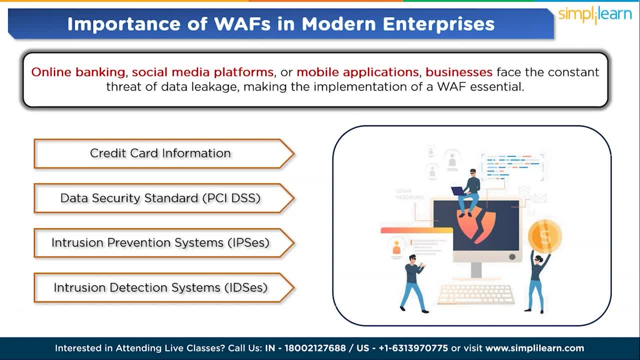 effectiveness of a WF is maximized when integrated into comprehensive security strategy. this strategy should encompass other security components like intrusion prevention systems, intrusion detection systems and both classic and next-generation systems firewalls. the synergy of these elements ensures a robust defense against evolving cyber threats in the dynamic digital environment. and now coming to 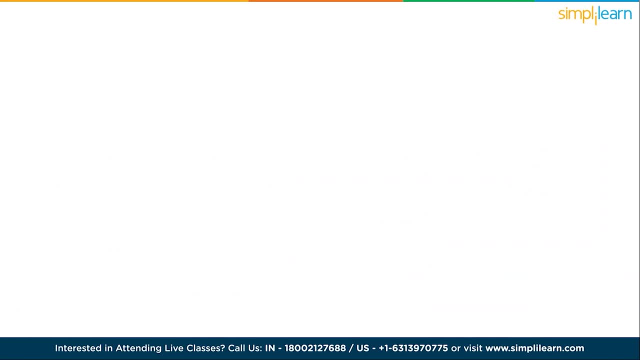 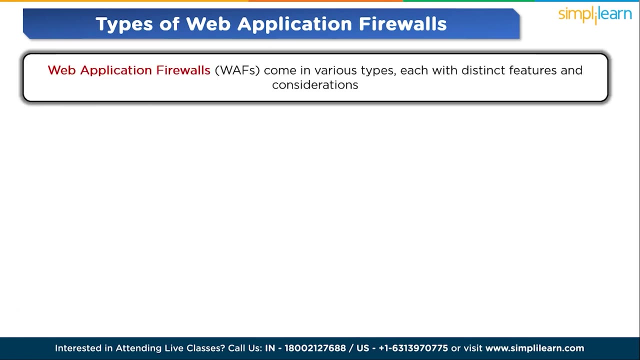 the types of web application firewalls and exploring the options. web application firewalls come in various types, each with distinct features and concentrations. let's delve into the three most common types. number one is network based WFs. network based WFs are hardware based solutions in stored lock. 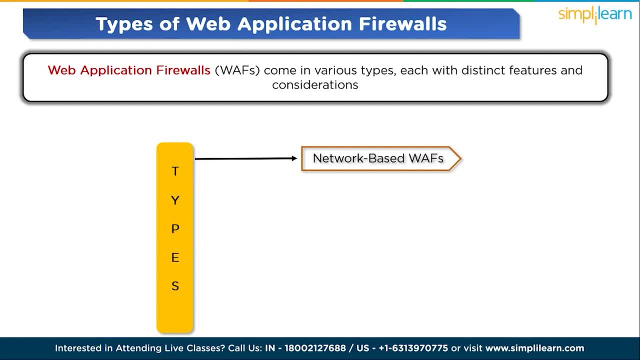 units, meaning a framework where small group of icing'll respond locally on premises through dedicated appliances. this proximity to the application reduces latency, enhancing performance, and major vendors facilitate large-scale deployment by allowing dual and settings application for ghosts multiple appliances. however, the drawback lies in the course upfront capital. 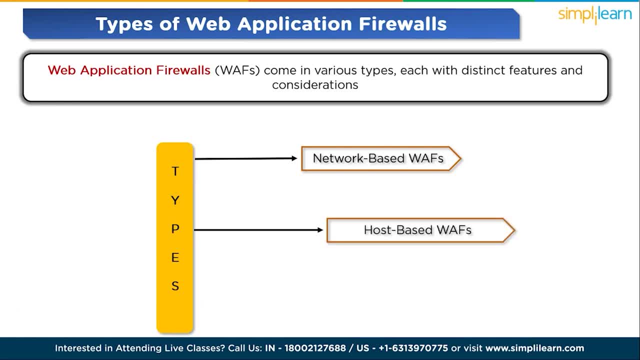 expenditure and ongoing operational expenses for maintenance. and then comes horse based WFs. horse-based WFs integrate fully into the application port. and now behalf two and they can be acquired through the server and decidin supply market right now. ここ coüyor dat sharing product nível上. 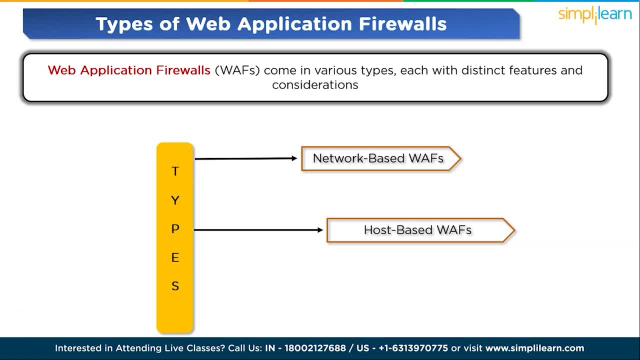 into the application port, offering a cost-effective solution with increased customization options. Despite their advantages, managing host-based WFs can be challenging. They rely on application libraries and local server resources, demanding more staff resources, including developers, system analysts and DevOps, or DevSecOps, for effective management. 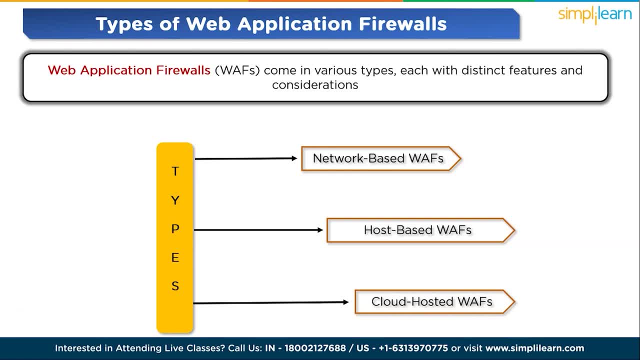 And then comes cloud-based or cloud-hosted WFs. Cloud-hosted WFs present a low-cost alternative, ideal for organizations seeking a chunky product with minimal management resources, Easy deployment, subscription-based models and simple DNS or proxy changes for application. 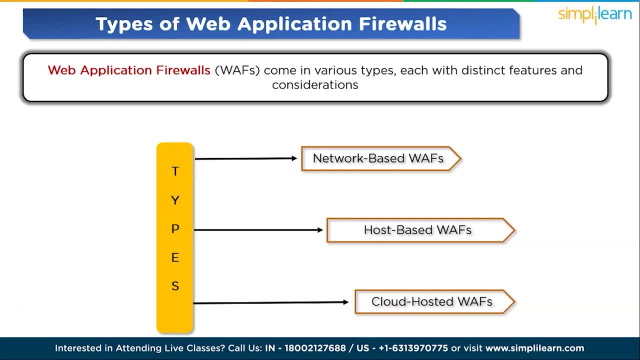 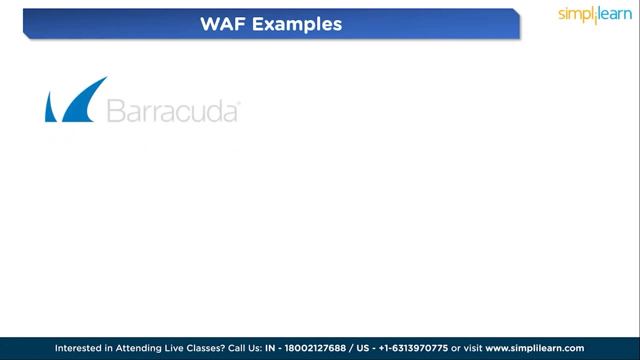 traffic redirection characterize these WFs. although entrusting a third-party provider with web application traffic filtering may pose challenges, It enables widespread application protection across diverse hosting locations. And now we'll see the WF examples: 1. Barracuda, 2.. 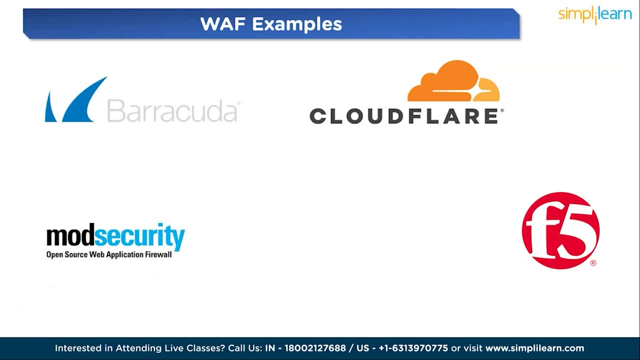 Cloudflare, 3. F5, 4. More Security, 5. Open Source Web Application Firewall, 6. NAX SI, 7. WebNite, 8. Open Source Web Application Firewall. And there you have it, guys. a closer look at the web application firewall, the unsung. 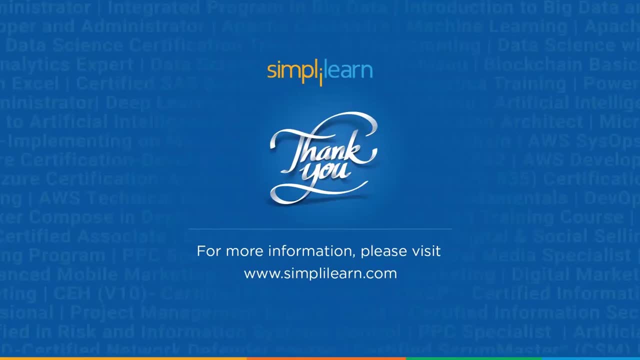 hero, protecting our web applications from various threats. If you found this video informative, don't forget to give it a thumbs up. Share it with your fellow digital explorers and subscribe for more insightful content. As always, stay secure in the vast digital landscape. 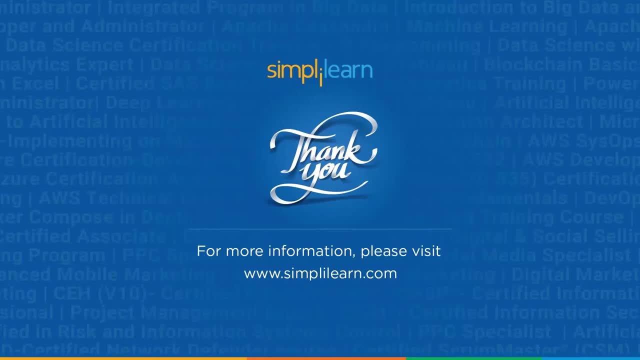 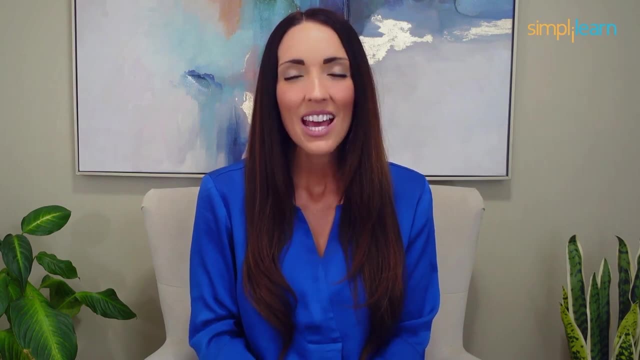 Now signing off, and until next time, keep learning and stay ahead. Staying ahead in your career requires continuous learning and upskilling. Whether you're a student aiming to learn today's top skills or a working professional looking to advance your career, we've got you covered. 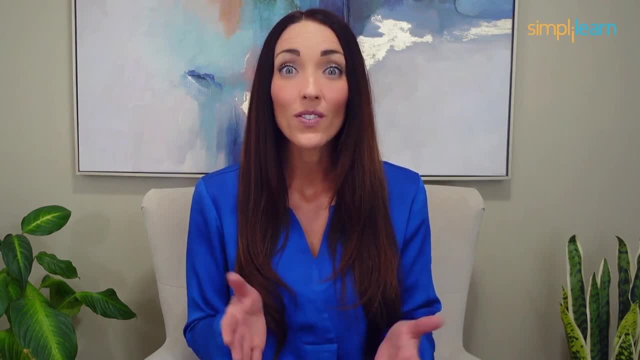 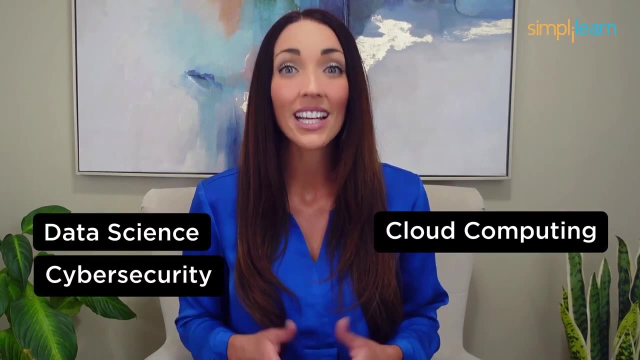 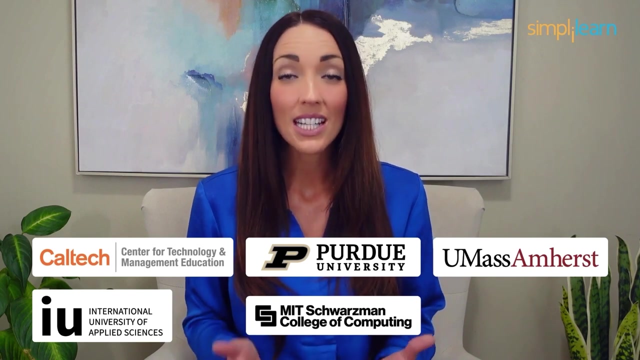 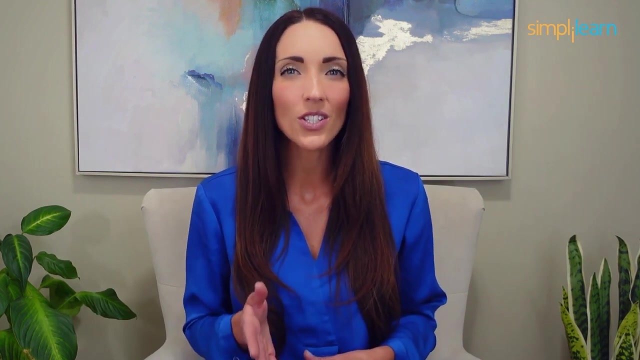 Explore our impressive catalog of certification programs in cutting-edge domains, including data science, cloud computing, cybersecurity, AI, machine learning or digital marketing, Designed in collaboration with leading universities and top corporations and delivered by industry experts. choose any of our programs and set yourself on the path to career success. 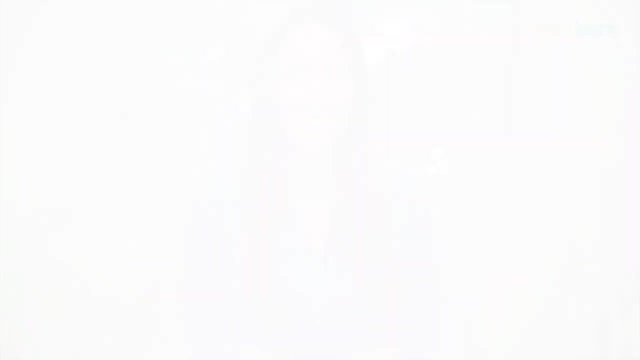 Click the link in the description to know more. Hi there, If you liked this video, subscribe to the Simply Learn YouTube channel and click here to watch similar videos. To nerd up and get certified: click here.